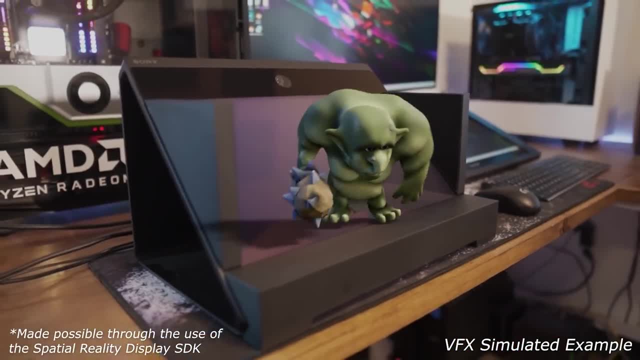 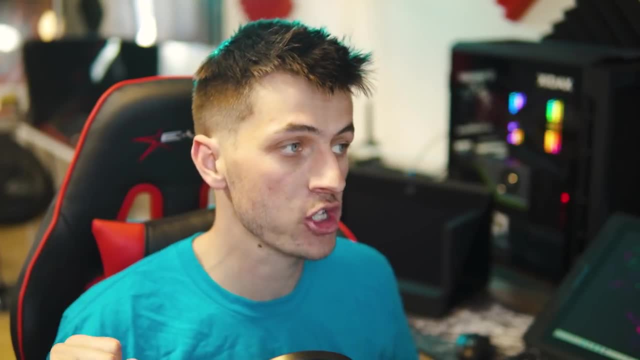 where I'll also use it to display our phone And I'll also be showing you the finished 3D animated character. so stay tuned for that, Alright, so for starters, on our character creation, we're going to need some reference, because it's really hard to just create something completely from scratch. 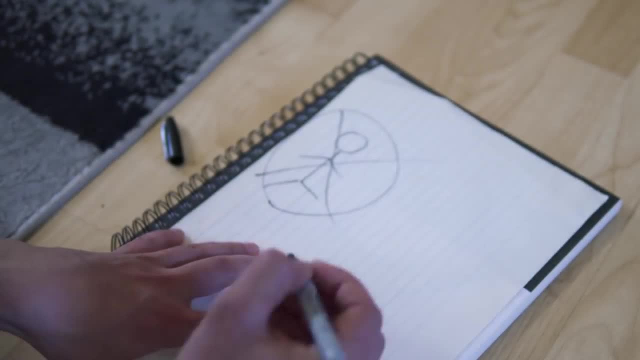 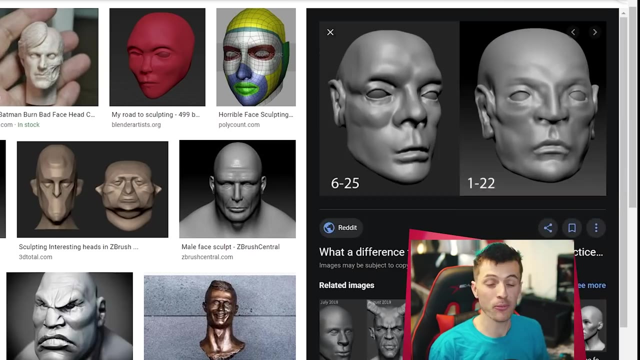 And I recommend not creating a human character right away, because it's really hard to sculpt the human face and really easy to tell when you don't have it right. This is a mistake I see a lot of beginners doing. You probably lose a little bit of confidence by starting with the human face and getting some hilarious results. 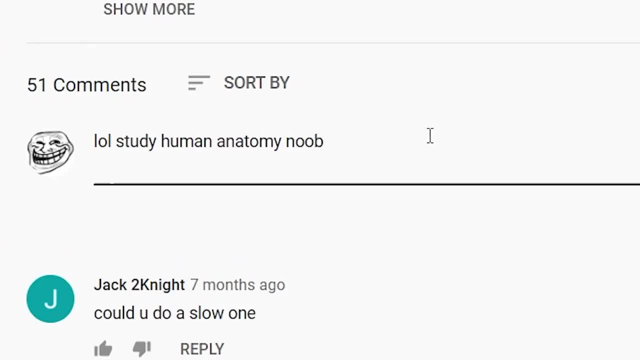 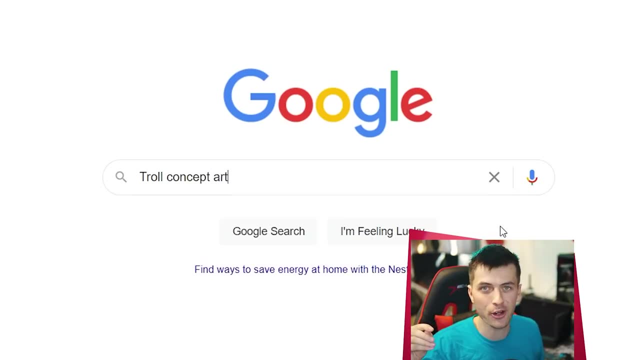 And if you try and sculpt the human head, chances are people on the internet are going to make fun. so I just kind of recommend avoiding that for your first few projects And coming back to it once you're comfortable with sculpting. So I recommend starting with a fictional character, like a troll. 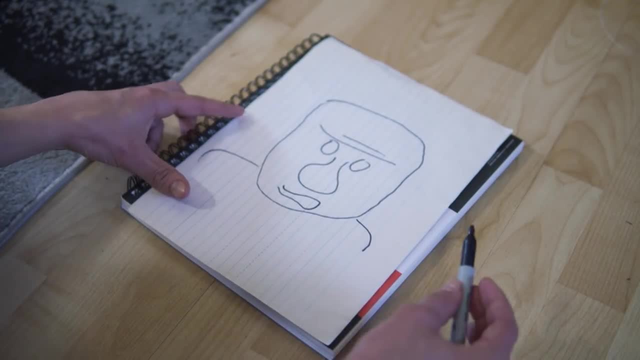 That's what we'll be creating today, And if you suck at freehanding with a pencil and can't draw, then I recommend using the internet to find some cool concept art For your concept slash reference art. I recommend using PureRef. 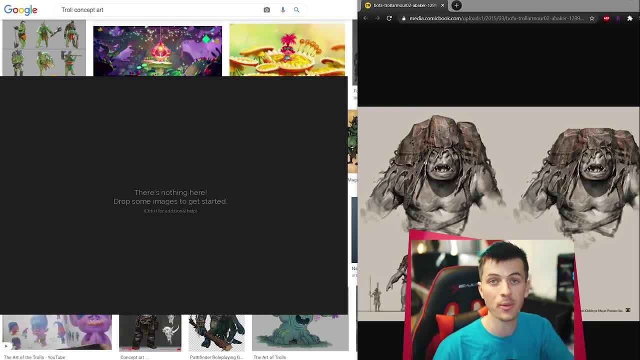 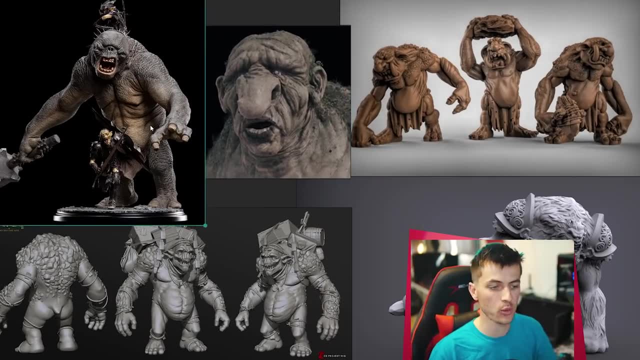 It's a really great free app that allows you to grab images off the internet and just throw them into a convenient window, And it's great for just grabbing random pieces of art where you might like something in one image or something from another one and just putting them all in one page where you can reference that then as you're sculpting. 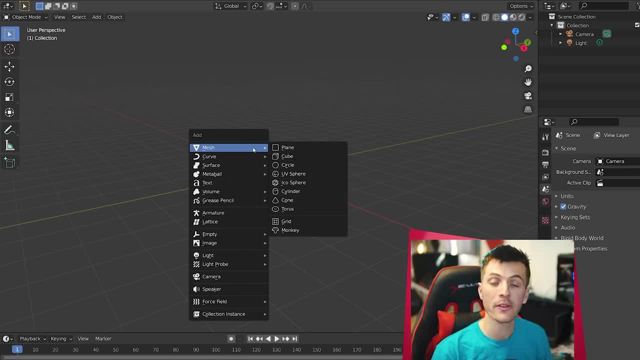 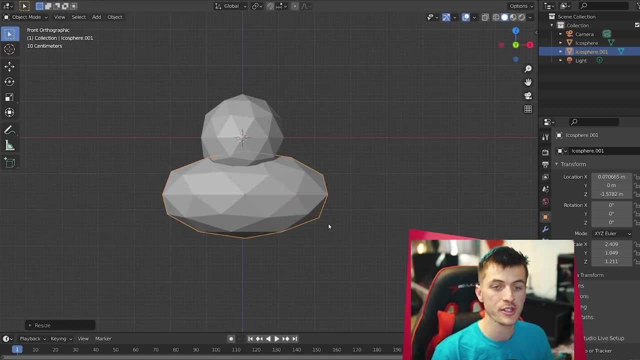 But now it's time to start blocking out our character For sculpting. so I like to start with a few primitive shapes, using an icosphere And just shaping it to the basic shape of a head, duplicating it and doing the same thing for some broad shoulders. 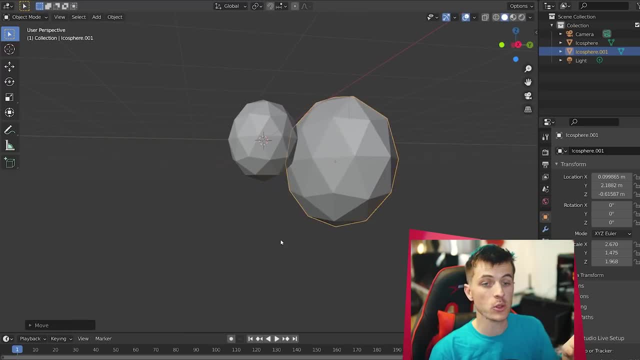 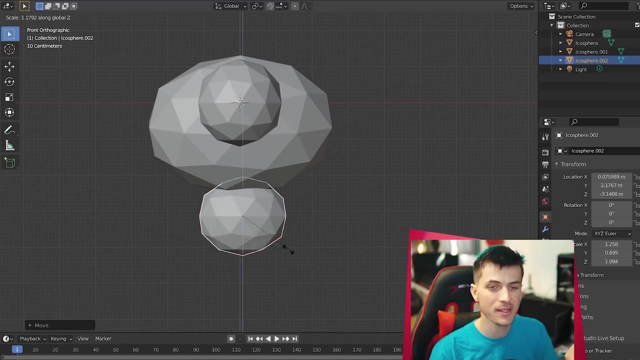 By doing this, we're creating a base mesh to sculpt off of, as well as getting sort of the rough proportions in order ahead of time. Just using Shift D to duplicate these icospheres and scaling and rotating them to kind of block out the basic shape of your character. 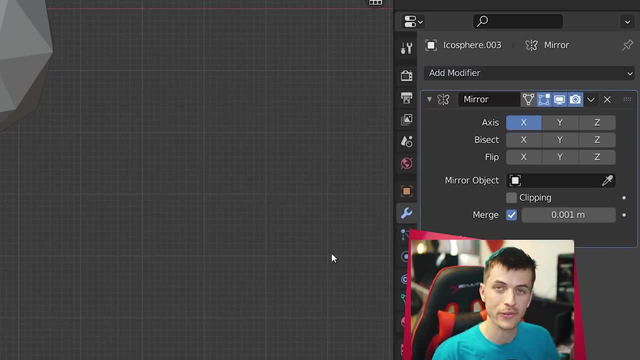 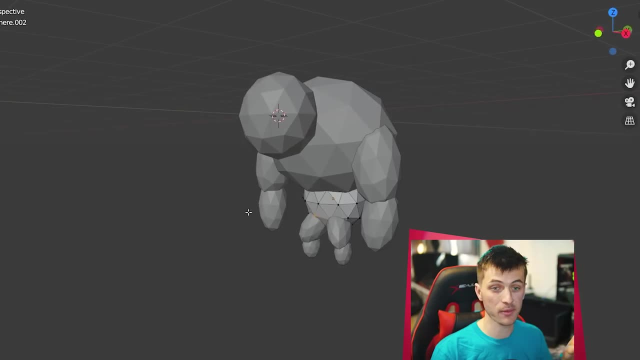 In this case a troll- And then you can use the mirror modifier and duplicate an icosphere in edit mode for the arms and legs. This just speeds up the process a little bit. Another tip is enabling proportional editing To kind of resize some of these icospheres to get the proportions you're looking for. 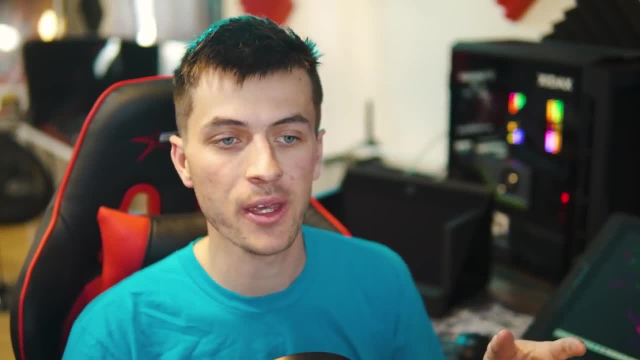 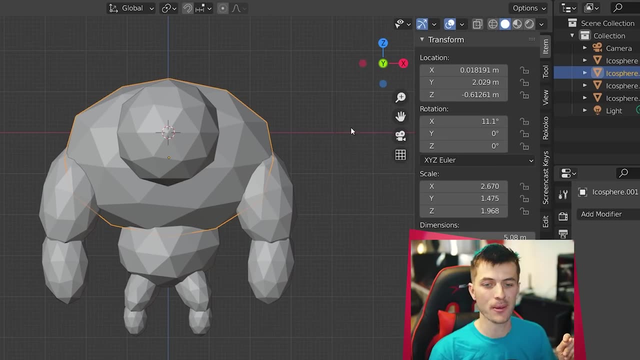 Now to combine all of these basic shapes together so you have an object you can sculpt on. you can go to preferences and add-ons and then enable the bool tool. This will allow you to have some really cool boolean options. If you hit N to bring up your properties tab and then go down to the edit button, you can see we have the bool tool options. 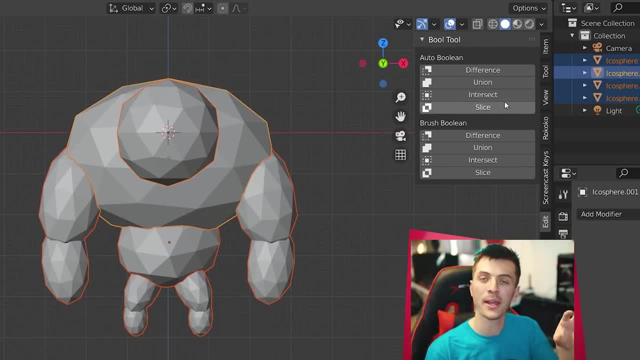 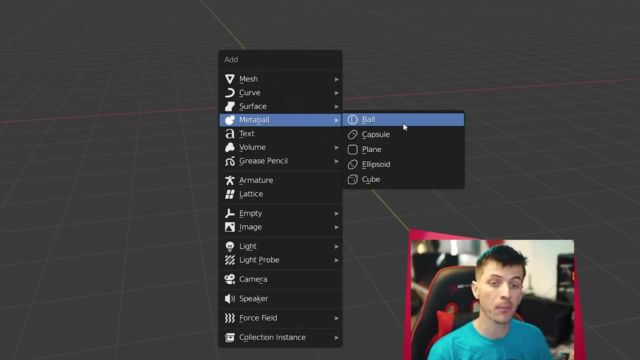 And if you select all of your primitive shapes and then just click union, it will combine it all into one single object where these are already connected. Another option for creating a quick base mesh to sculpt on is using metaballs. You can go ahead and add a metaball. 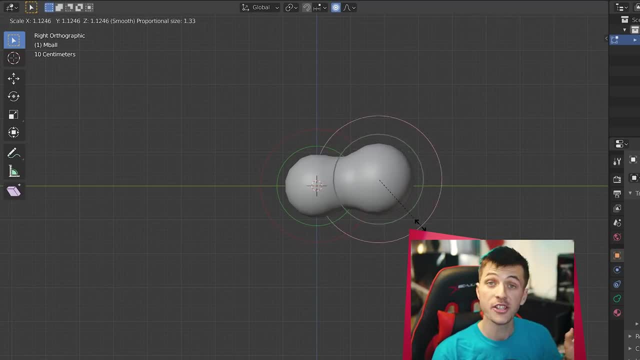 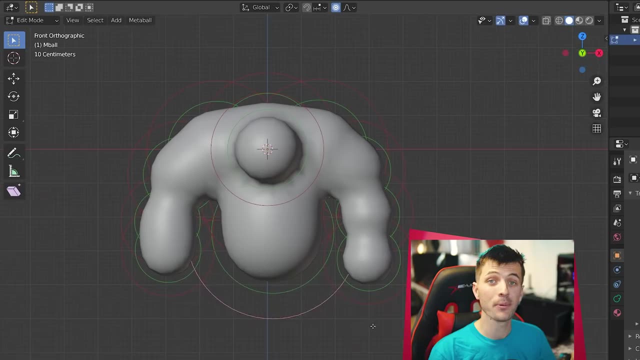 And then just tap into edit mode and start duplicating this with shift D. And this is just another option where you can keep duplicating these metaballs and scale them in different ways to create a blocky shape that you can also sculpt on. This is just a lot of fun to play with and another option that is commonly used, so I thought I'd mention it. 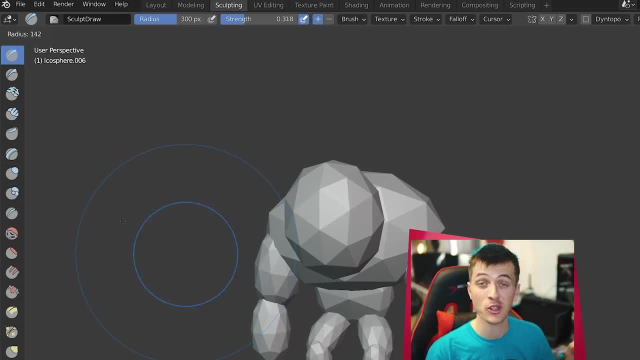 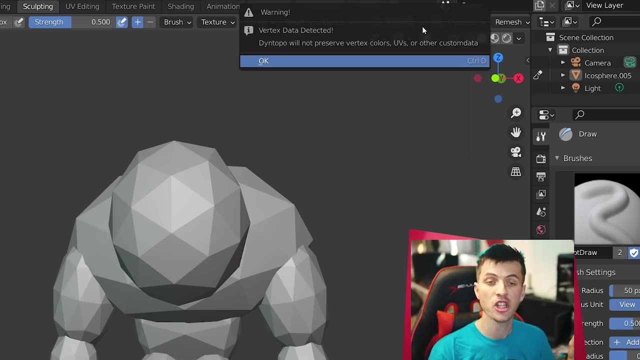 So now you can switch to the sculpting tab and start adding in some light details on your base mesh. A few shortcuts is F to change your tool size and shift F to change the strength. Also, you'll probably want to enable dynamic typology by clicking that up in the corner. 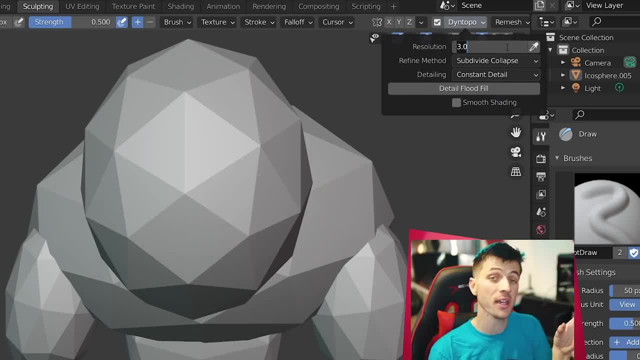 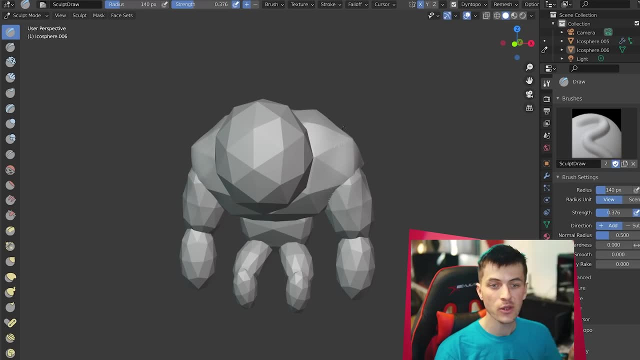 I like to change the detailing to constant detail and I found a detail size of 12 to work well. Starting with the draw tool and enabling the X mirror option so it mirrors your sculpt on both sides of the mesh, You can start blocking out some basic muscle. 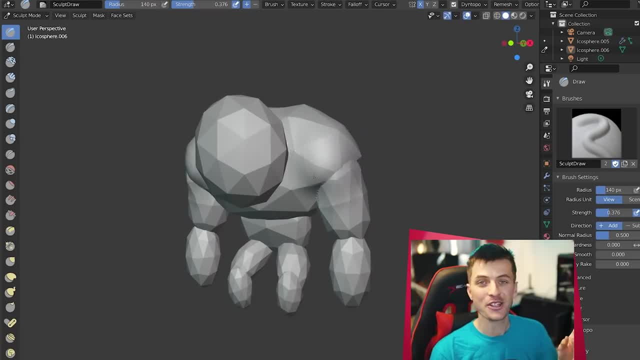 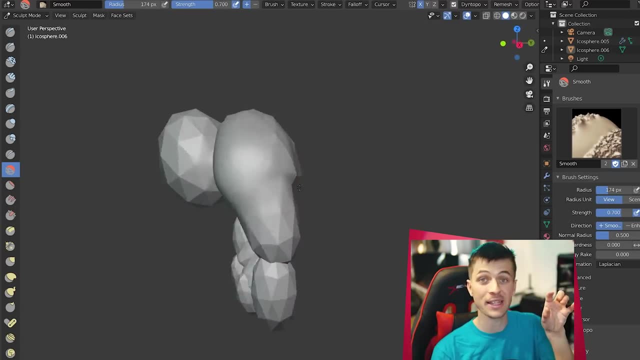 Muscle, Some basic muscle structure. You can start sculpting out some basic muscle structure. Then we have the smooth brush. I use this to just go back and smooth over all my mistakes. Anything that looks bad, it's basically an eraser for it. 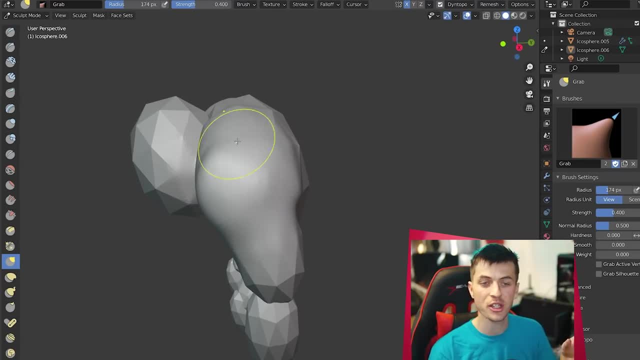 Next we have the grab brush. This works exactly like it sounds. You can nudge around the mesh and kind of pull things into shape, More or less like forming something with clay. It's really handy to fix those little mistakes and tweak things. 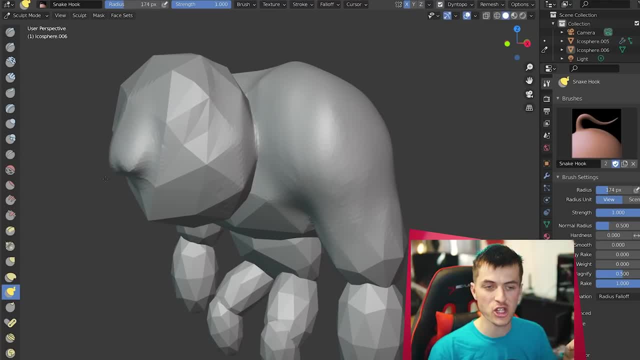 Then I like to use the snake hook. This one's a lot of fun for adding extra mesh to the scene. For example, like the nose on a character, you can just pull out a chunk of geometry Adding more mesh and detail to that specific area. 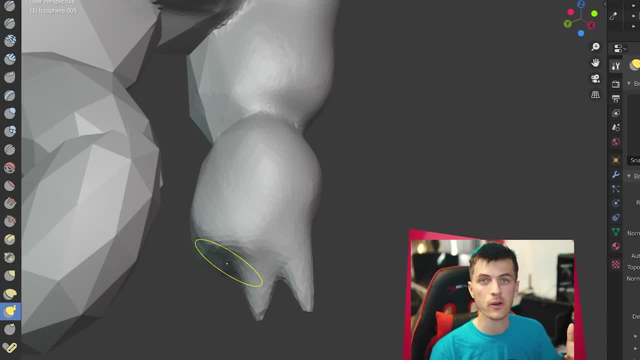 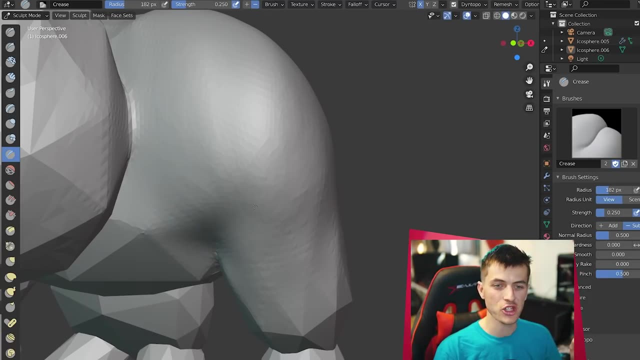 This also works great for things like the feet on a character or the fingers. Where you don't have any base mesh to work off of, you can pull out the more small detailed geometry. Then there's the crease brush. This works great for adding definition to the muscle structure on your character. 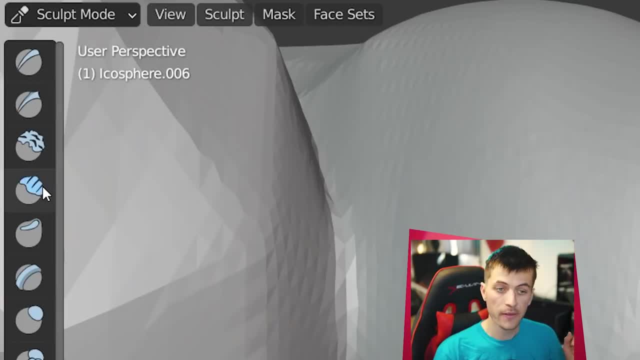 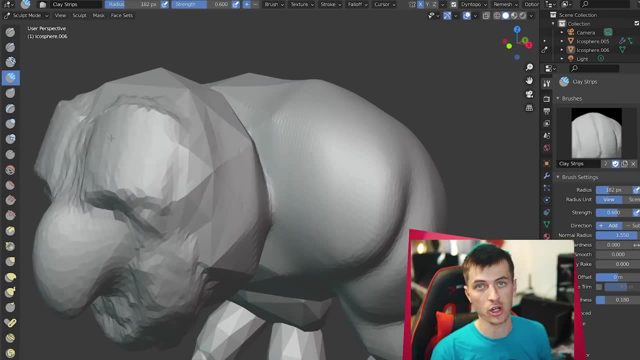 It just works great for shaping out the muscles on the arm or chest of a character. Then there's clay strips. This works great for just adding extra geometry again to your scene, Filling out an area in the face or something where you need more geometry to work with. 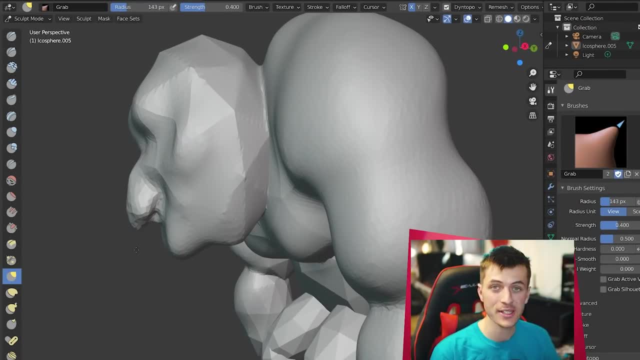 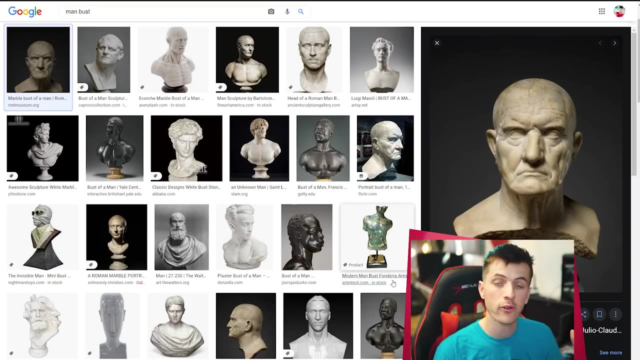 But now it's time to just go to town on your model, using these tools to create the character you're imagining. Even if you're not creating a human character, I still recommend getting some reference art of the human structure online for the muscle systems and stuff. 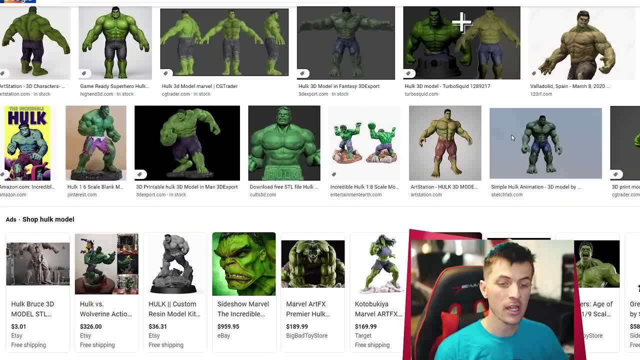 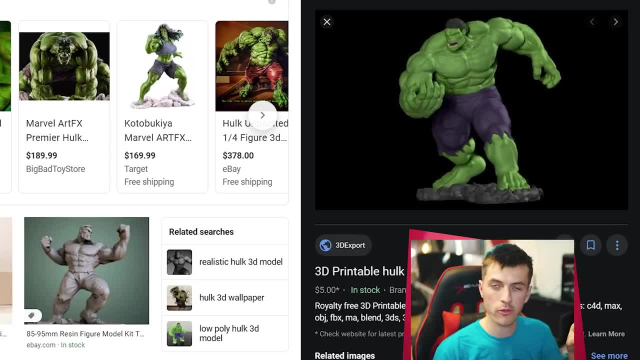 Because that is something that will be kind of universal in any character, And so for this I used some reference images of like the Hulk, for example. Using this sort of reference art is helpful to me to just make sure that I'm getting the muscles in sort of the right places on the character. 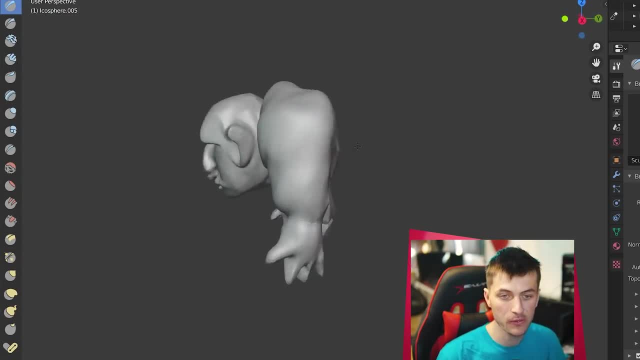 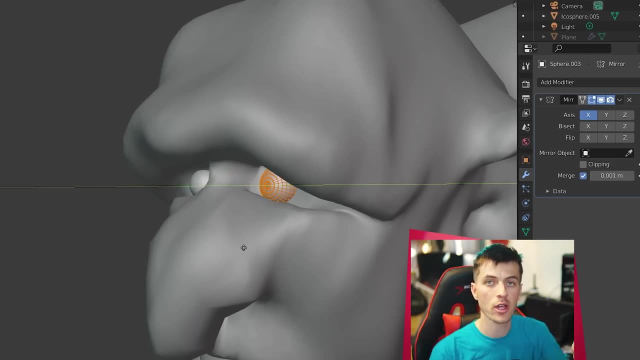 Otherwise it can look unnatural. But go to town having fun with these tools in combination. Once you're getting pretty happy with the character, you might want to go ahead and add in some UV spheres for the eyes. This will give you some geometry to sort of work around in your sculpting. 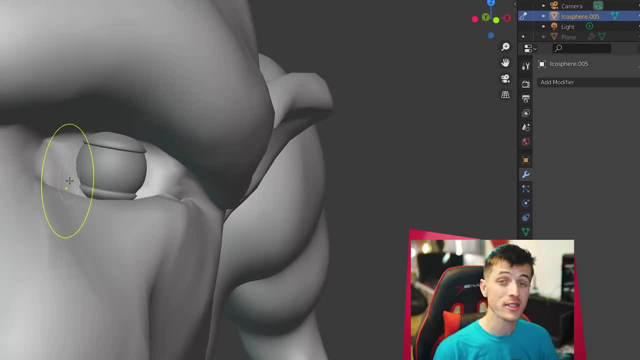 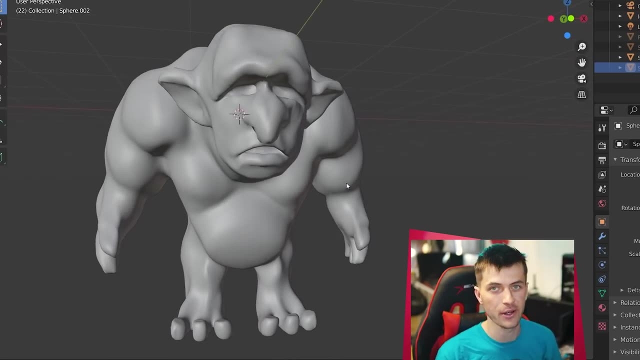 Sculpting out the base mesh of your character. It might look pretty hilariously bad at times, but the more you add detail to your character and continue to just tweak it the way you imagine it, The more you'll finally get something that you're pretty satisfied with. 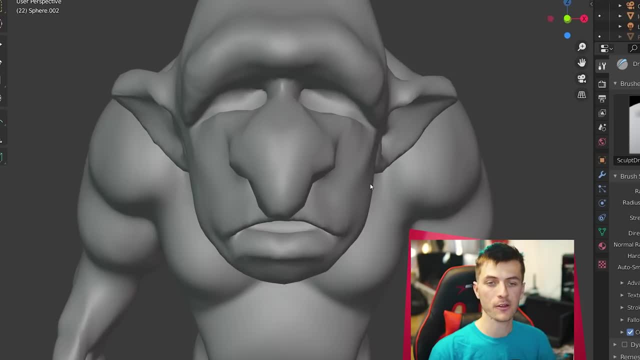 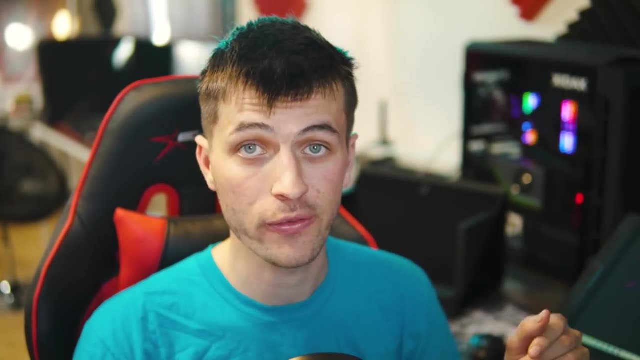 A few hours later And look at that, we have a basic character that doesn't look too terrible. It could be something like a clash of clans or clash royal character. But now it's time for the next phase in the character creation workflow, And that's retopology. 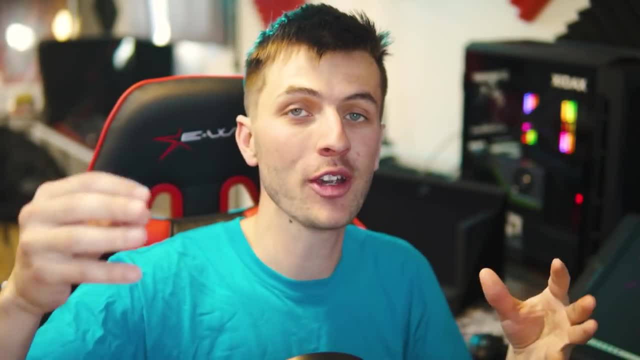 So if you don't know what retopology is, it's basically going over now and recreating your mesh that you have roughly sculpted out in a clean fashion, Starting by adding in a basic plane and moving it to the right in edit mode. 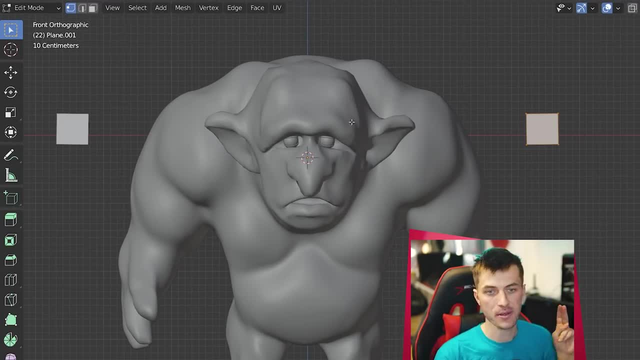 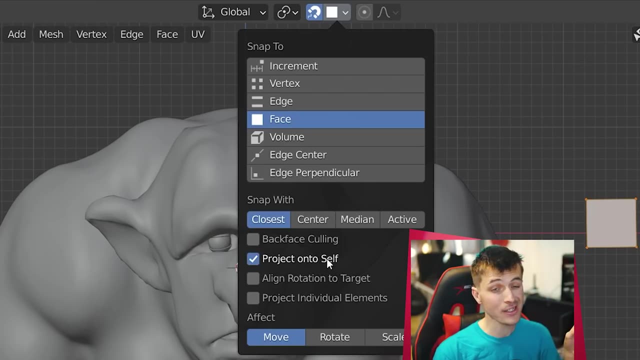 We can now add a mirror modifier. so we're doing this twice as fast And along the top bar we're going to enable snapping. We're going to choose snap to face, And then we're going to also choose project onto self, Back face culling. 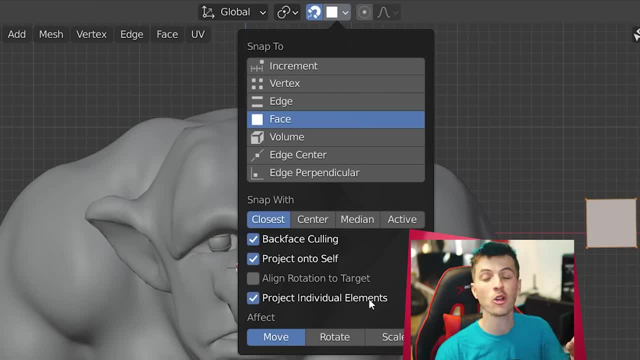 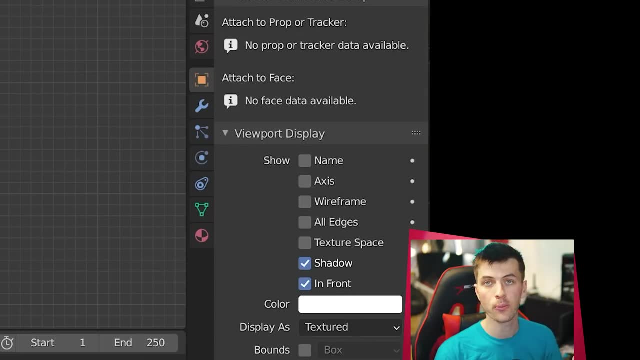 And then project individual elements. This will make it so your mesh will automatically snap to your sculpted mesh as you're working over it. Also, with the plane selected in the object settings you want to enable in front under viewport display, So the mesh doesn't get hidden inside of your sculpted mesh. 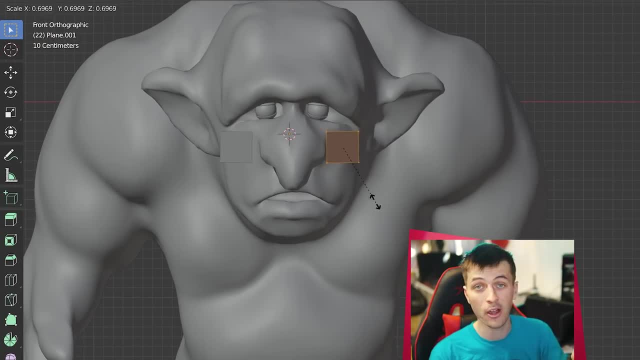 Now, if you place the plane over the character, you can see it's already being meshed to the shape of the underlying mesh. We're just going to scale it down nice and small, and add in one more modifier. That's going to be the shrink wrap modifier. 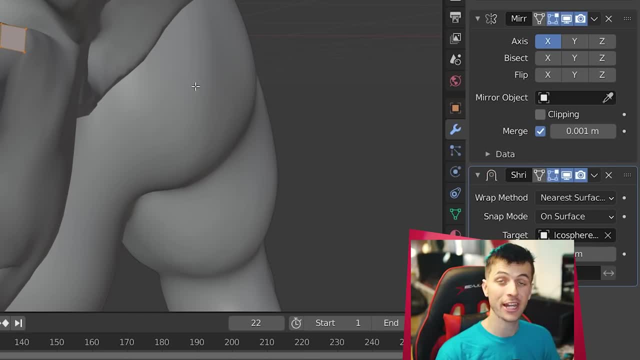 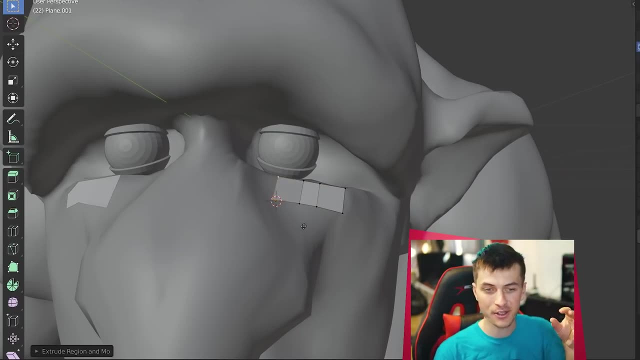 We'll choose a target of the underlying sculpt mesh And this will just add to the accuracy of how well that mesh will snap to the underlying mesh, making retopology manageable. Now you can just grab a few vertices and start extruding out that mesh and it will be snapping to the underlying sculpt mesh. 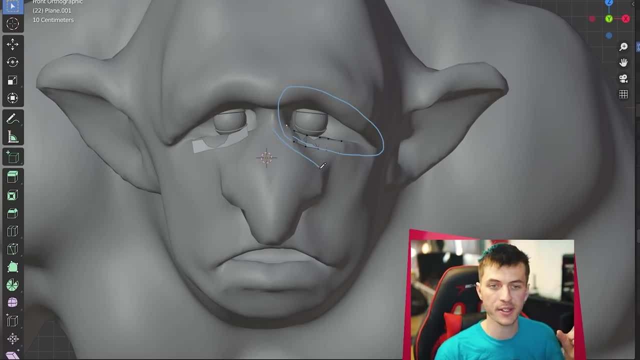 Now typically for retopology. you want to make sure you have some nice rings of vertices around your character's eyes, nose and mouth. This makes for the cleanest geometry for animating and deformations in the face, So you don't get any weird jagged shapes in the face while it's deforming. 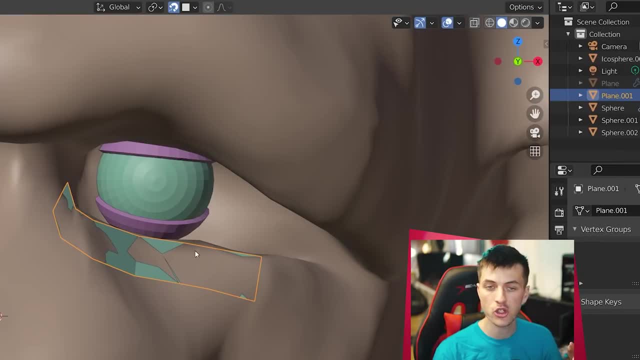 A quick tip to help identify what object you're working on is under viewport display. choose random And that will give each object a different color in the viewport. So now it's time to just start extruding and adding geometry in the shapes we were just talking about. 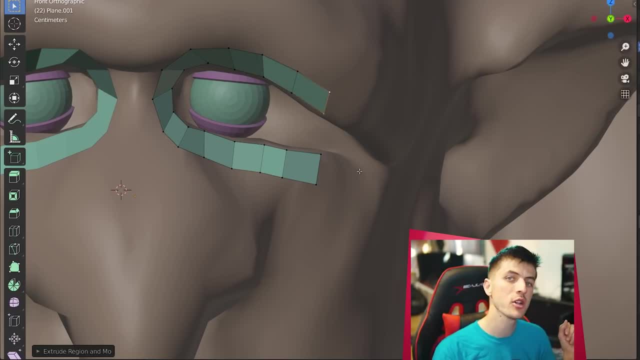 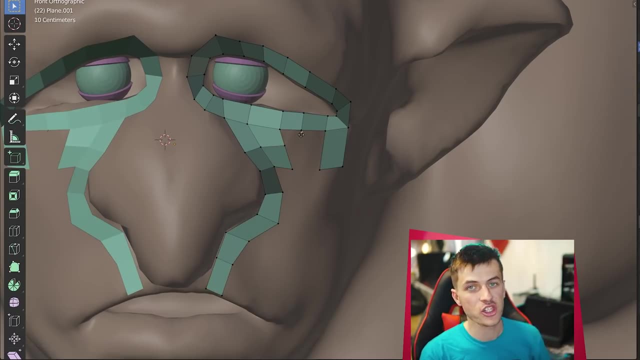 This is where it can get a little tiresome. So you want to put on some of your favorite music and just make a game out of it, Keeping the geometry clean and only using faces for the cleanest deformations, Mainly just extruding the geometry with E and then connecting the four faces with the F key. 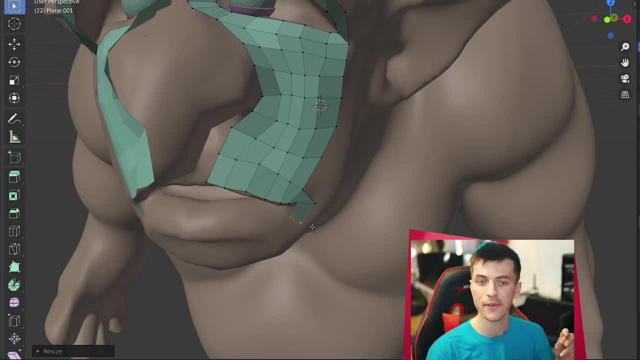 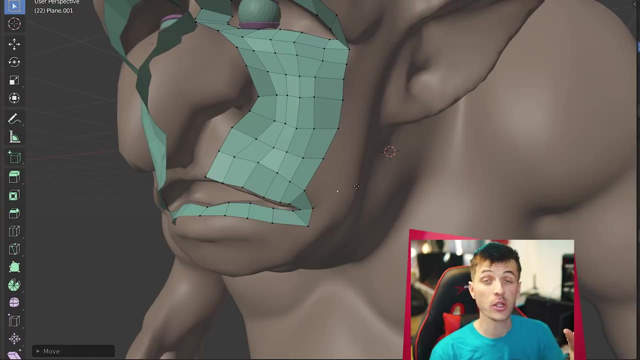 Another shortcut is when you have two vertices selected, you can hold control and left click to extrude geometry out really quickly just following the mouse cursor. Also, you want to make sure you check clipping on your mirror modifier. Then just go to town filling out your character as clean as possible with these faces. 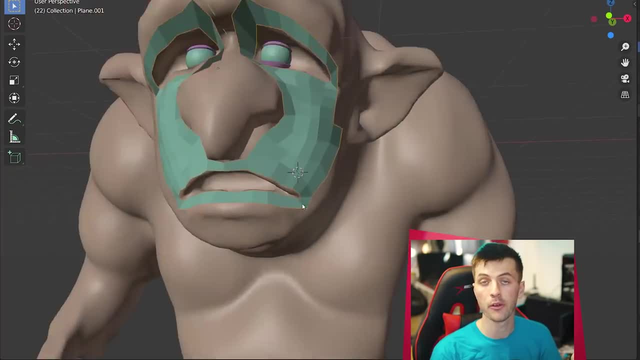 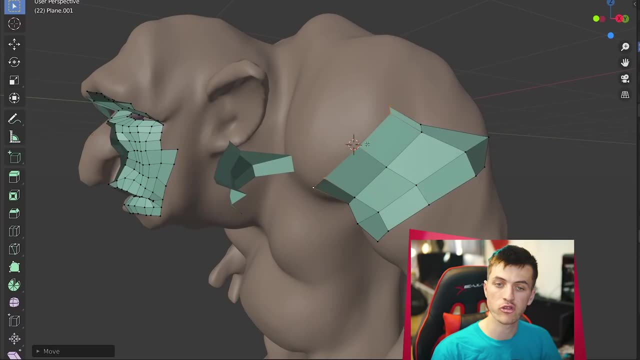 Following the flow of the mesh, with circles around them, Around the mouth, nose, eyes and ears, Areas like the arm. here you don't have to add as much geometry because there's less detail, So you can get away with larger faces and extruding more at once to make things go a little faster. 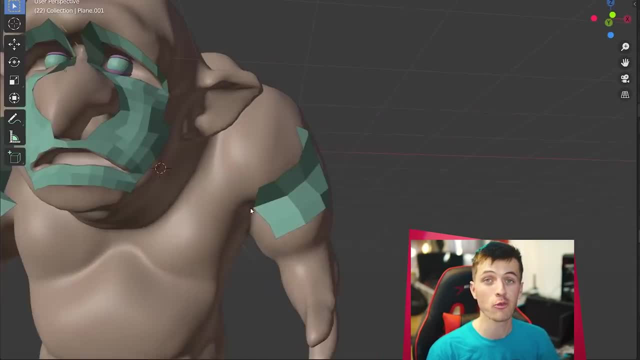 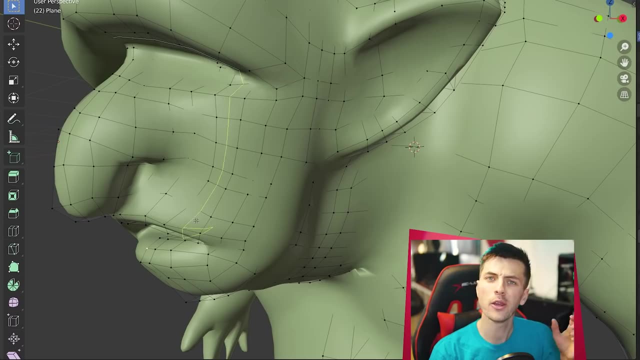 But fast forward another hour or so of listening to your favorite music and having fun, retopologizing, And you should have a mesh looking something like this: And at this point you can add a subdivision surface modifier to your mesh And then you can add a little bit more detail to the geometry where you want more definition in your model. 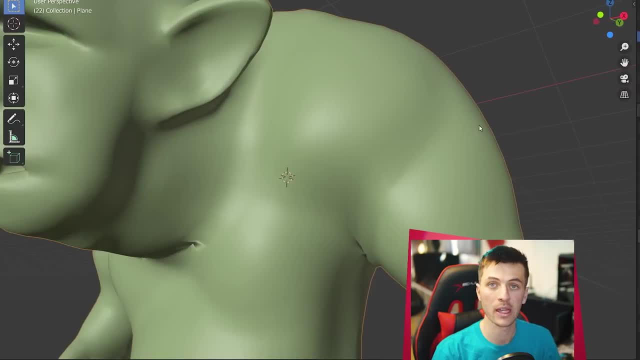 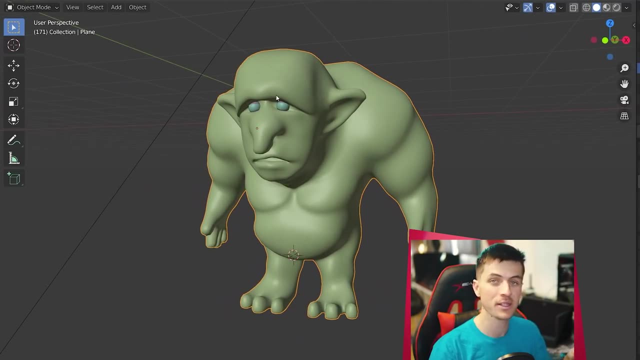 For example, you might want to add more vertices around the mouth or muscles, To kind of add more definition as well At this point. so it's not too smoothed over. Now that you have your character sculpted and retopologized, The next step would be to add a texture to it. 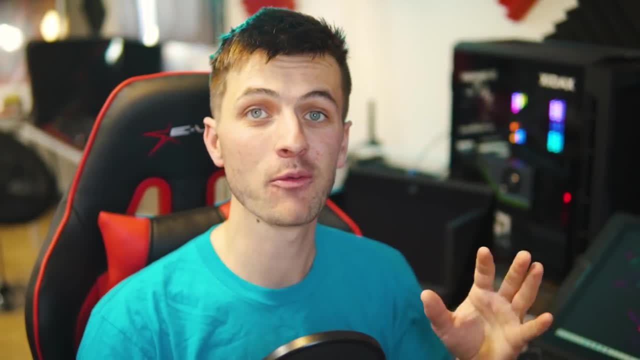 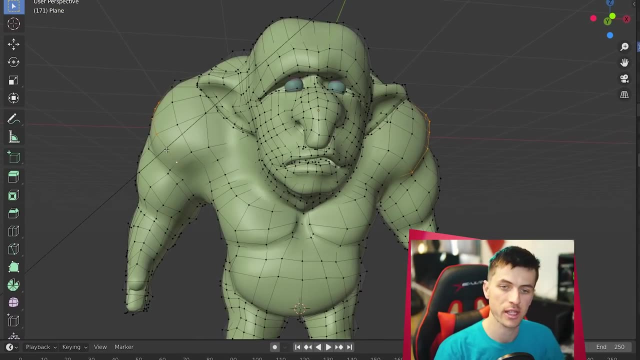 So for this, we first need to unwrap it. This is essentially so. we can put a 2D texture over a 3D object. So for unwrapping, you're going to select rings of vertices around the limbs of your characters, Like the arms, for example. 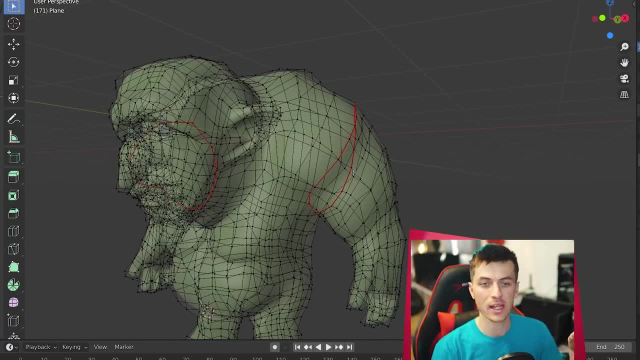 And then if you go control E, you can mark a seam And this will be where we can kind of cut the mesh there when we unwrap it, So we can separate the arms from the body, from the head etc. Typically you want to kind of hide these seams. 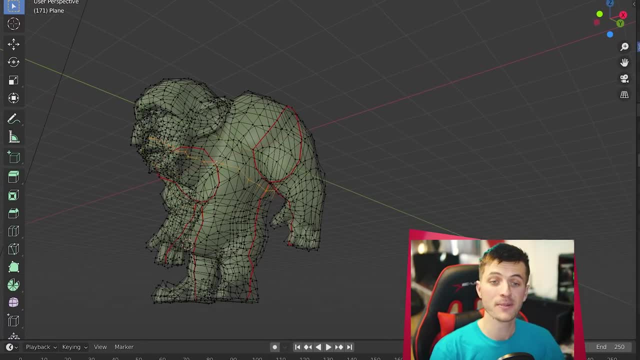 So I'm going to add it along the side of the mesh here as well, Just adding seams to the other areas of the mesh, like the ears and neck and stuff, So we can separate all these different sections and we'll get more detail then in our texturing. 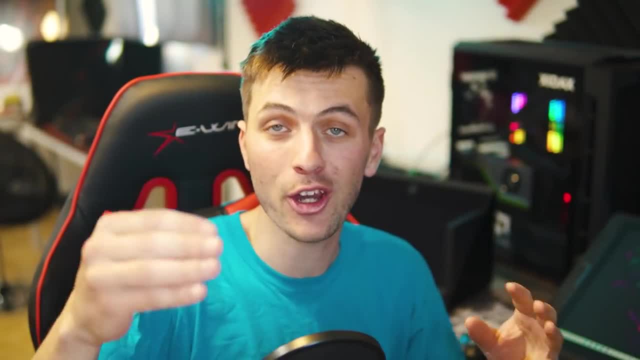 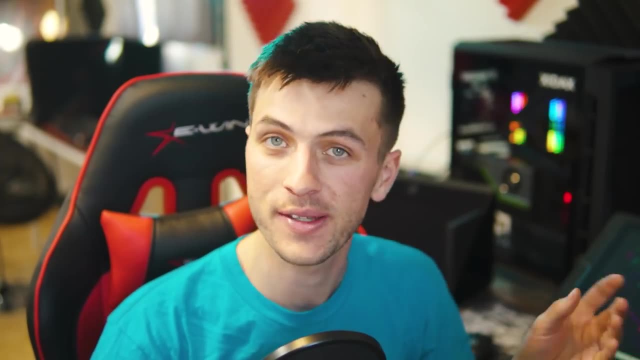 A good way to explain UV unwrapping is essentially: think of wrapping your character now in wrapping paper. And how would you cut that wrapping paper if you wanted it to fit on the character? That's essentially what we're doing with the seams. So now in the UV image editor you can create a new image. 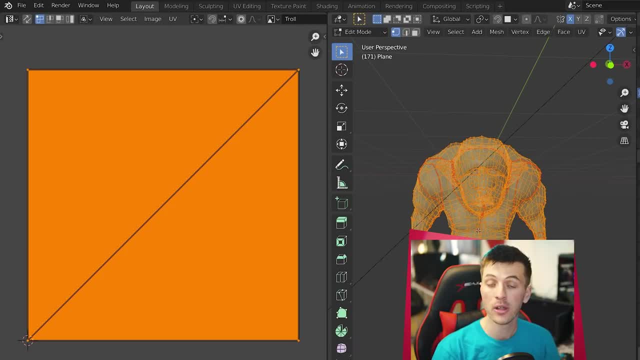 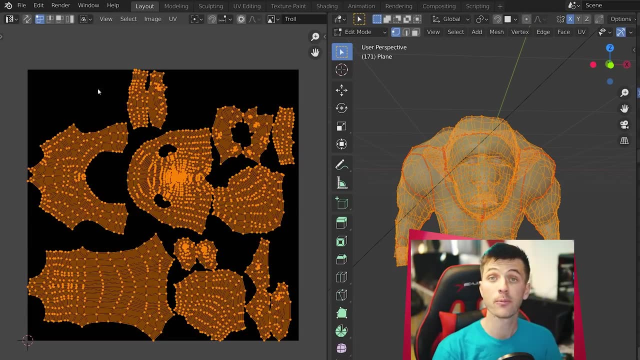 We'll just give this like a 2K resolution And then if you tab into edit mode, hit U and choose unwrap, You can see we have all the separate pieces now of our mesh laid out on this 2D image. A few tips for improving this is choosing the minimize stretch option and the pack islands option. 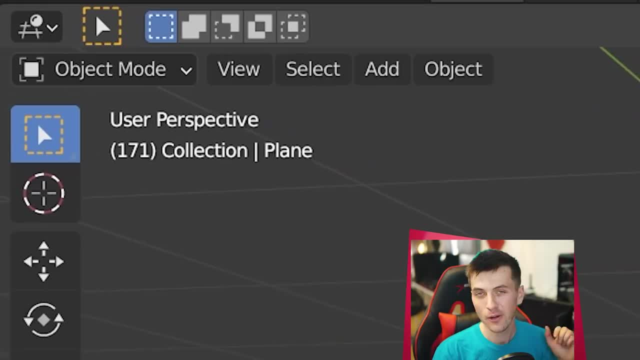 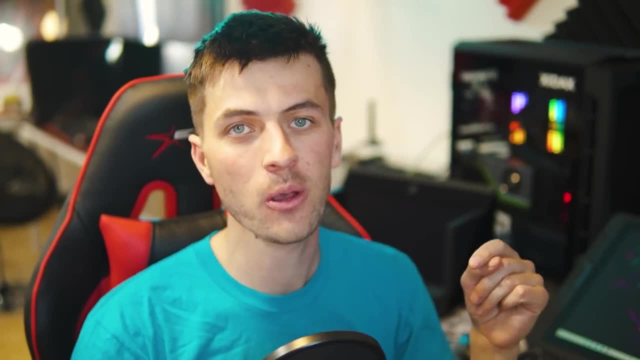 Just to get the most resolution out of that texture as possible. Now for the texturing part. you can either do it through texture painting or vertex painting, Or you could use a third party application. But we're doing this all in Blender And we're keeping this character sort of simplistic. 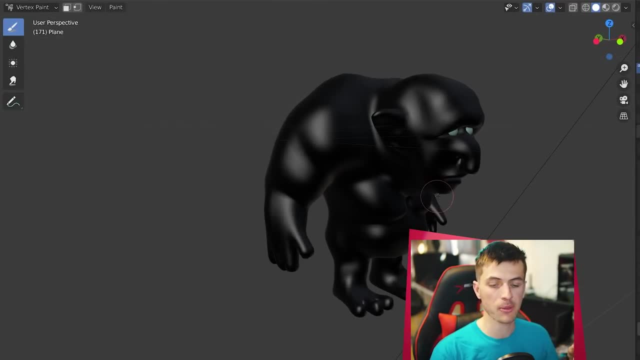 So I'm going to go with vertex painting for this character, Because it fits the theme that I'm going for and it has a few tools that will make it really easy. So, switching from object mode to vertex painting. You can see our character currently doesn't have any color on him. 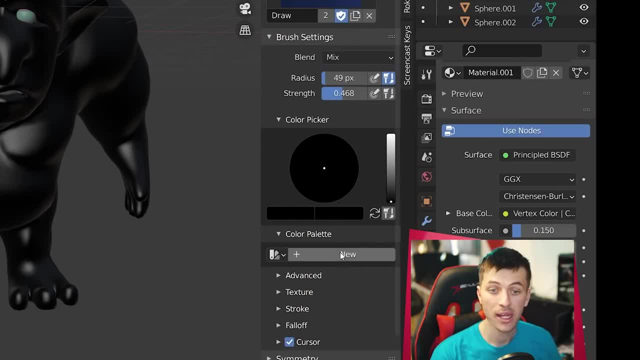 What you want to do is hit N to bring back your properties tab And create a new color palette. Here you want to choose some of the main colors that you'll be using for your character And then just hit the plus key to add them to your color palette. 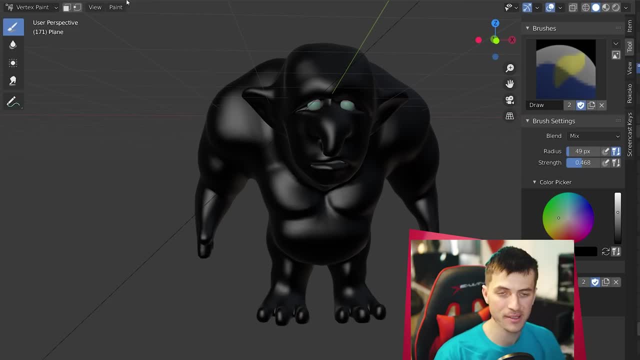 This will keep it easy to grab those colors later. I like to start by picking my base color and then choosing set vertex color to make the character all that one color. Sometimes you might want to play around with a few different colors until you find something that you're happy with. 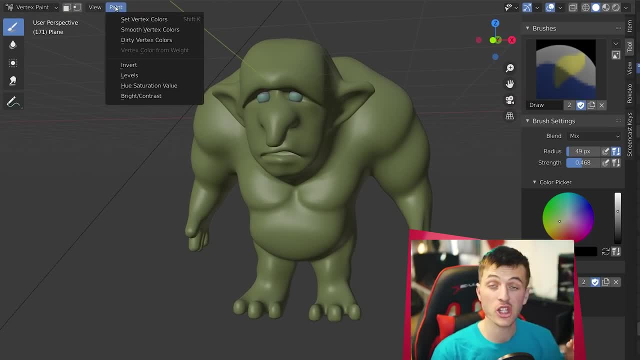 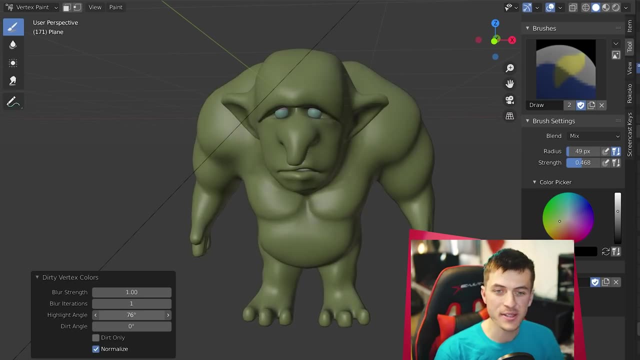 Then I'm going to use a feature called dirty vertex colors to make shading on this character really easy. If you use dirty vertex colors And then choose a highlight angle of something around 90. You can see that this does a whole lot of shading already for us in the crevices on the mesh. 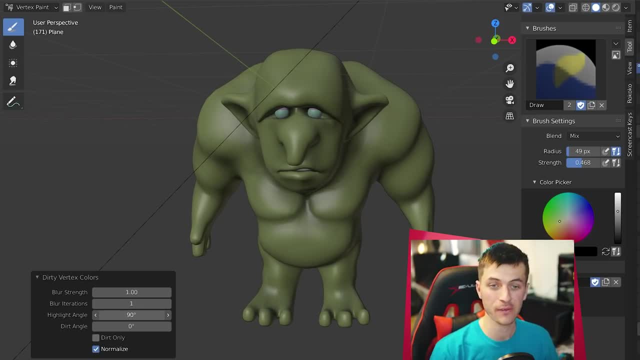 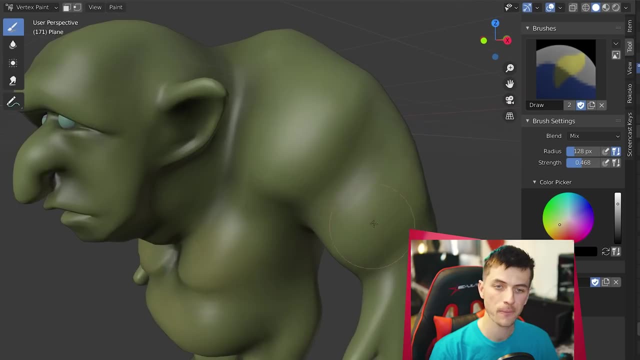 Giving it that really cool shading that you might want on a character like this, And it saves just a ton of time by doing this automatically. Next, you might want to grab a lighter skin tone and start painting some highlights over the character, Basically just going to the more fleshy areas of the character and adding a lighter skin tone. 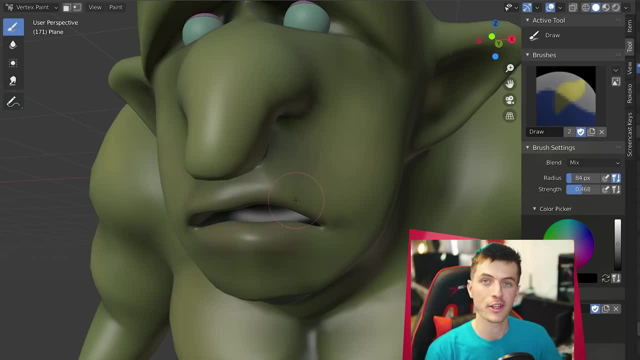 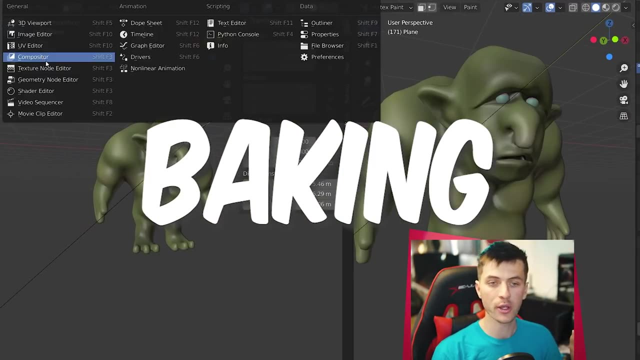 And then you can also do the same thing with a darker color to kind of fill in crevices. But once you're happy with your vertex painting, We'll want to bake that to a 2D image texture, So you can just switch to the shader editor in a new window. 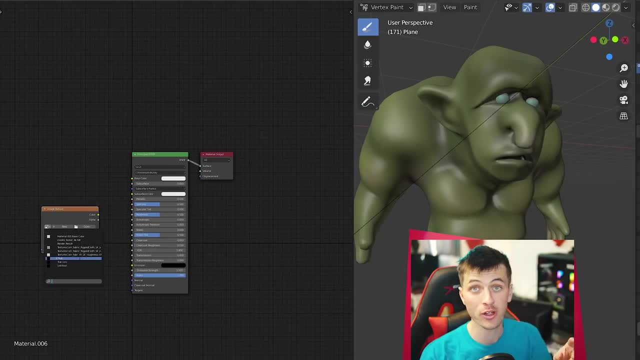 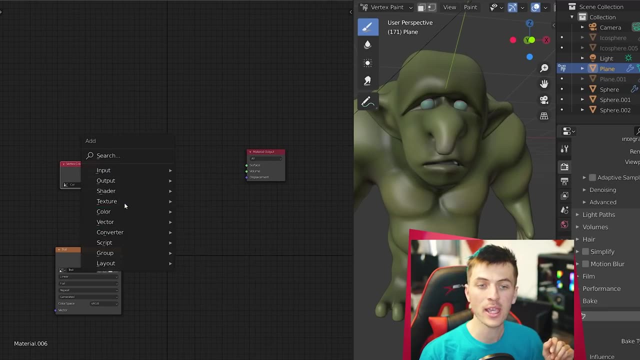 And here add in an image texture And select the texture that you created in the UV editor. You want to add in one more node and that's the input vertex color. Here you'll want to select the color that we just painted And then, if you add in an admission shader, 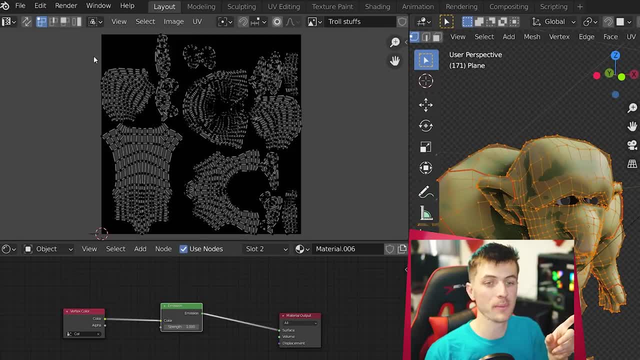 And connect the color to the color and the output to the output. And then you'll also want to make sure that you save the texture you created in the UV editor out onto your hard drive. And then for baking you're going to have to use cycles. 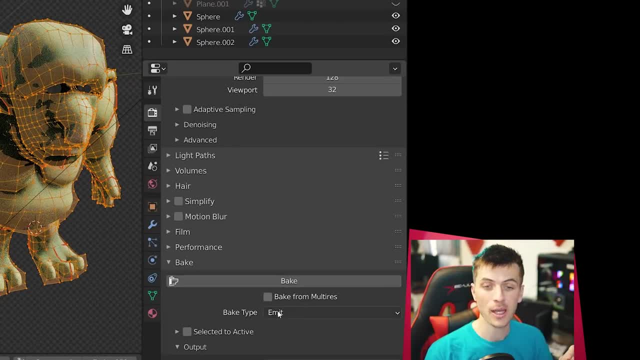 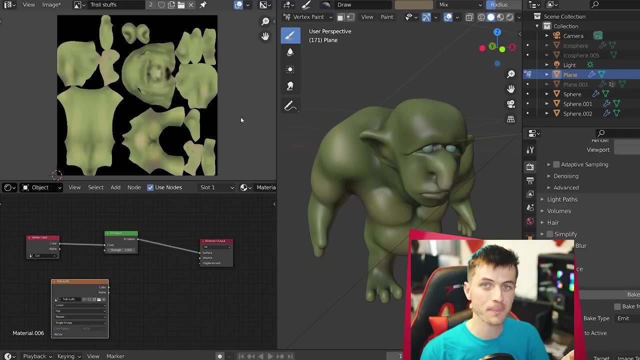 So change the render engine from EV to cycles. Scroll down to your bake options And make sure you have the bake type set to 0. To emit: Once you have that set, all you have to do is click bake And then you'll see that we get that vertex paint baked onto a 2D image texture here. 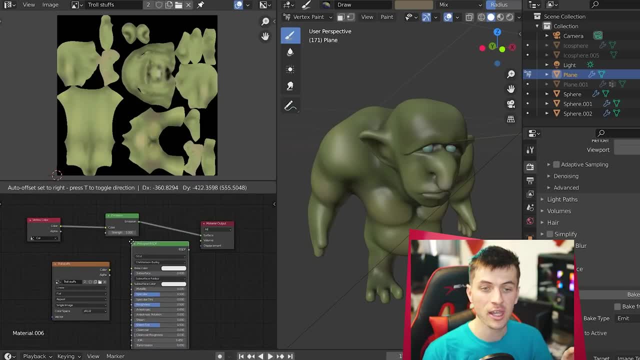 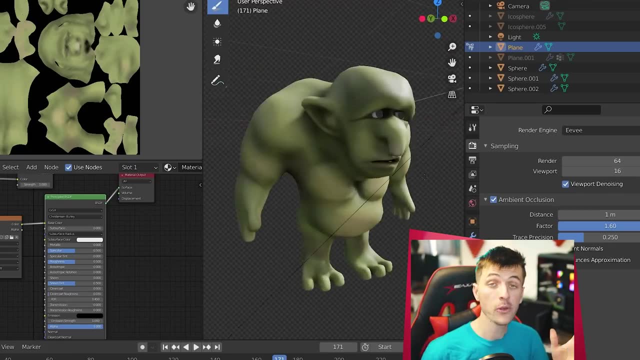 You can go ahead and save that now And then add in a principled shader again, Connect the color up here And use that as the output. And there you can see in the EV rendered view that we now have our character textured. A few quick tips to improve the material a little bit. 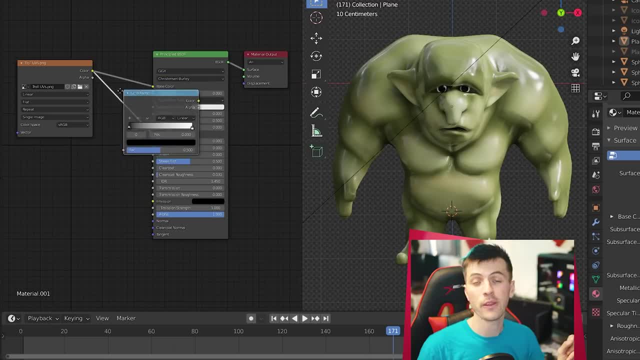 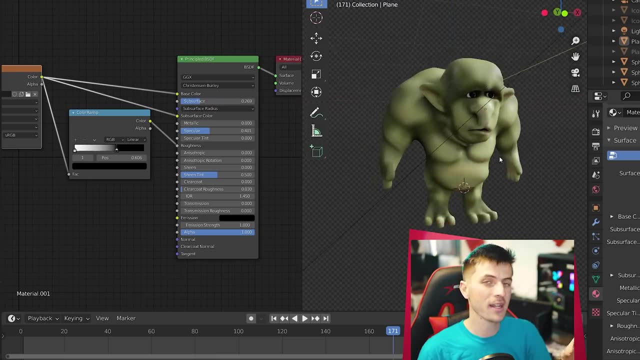 Would be connecting the image texture to the roughness, Adjusting the value a little bit with a color ramp And then also using the image texture as the color for the subsurface scattering And giving it a little bit of subsurface scattering, Just to add a little bit extra to your renders. 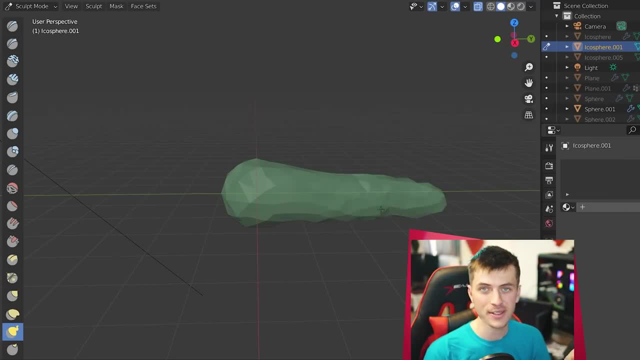 But now it's time to accessorize your character. This is a good way to add a little bit of extra detail And give him some personality. So what I did is I sculpted a basic club using an icosphere And then mainly using the snake hook tool to pull out extra geometry. 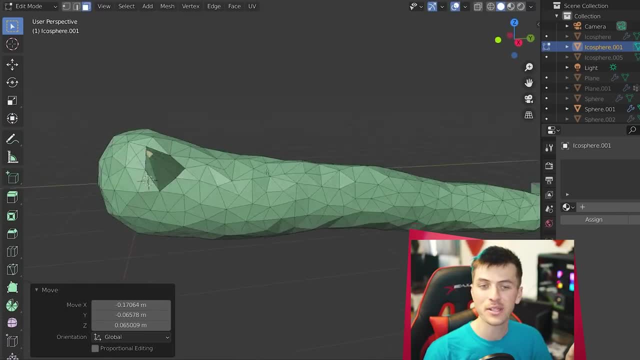 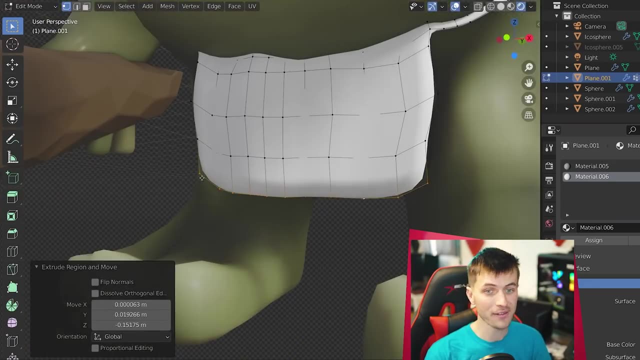 Then I just extruded out some spikes onto that icosphere, Gave him a different material, Along with a little bit of vertex painting of its own. Of course, your character also needs clothes, So, duh, Don't forget to add something for that. 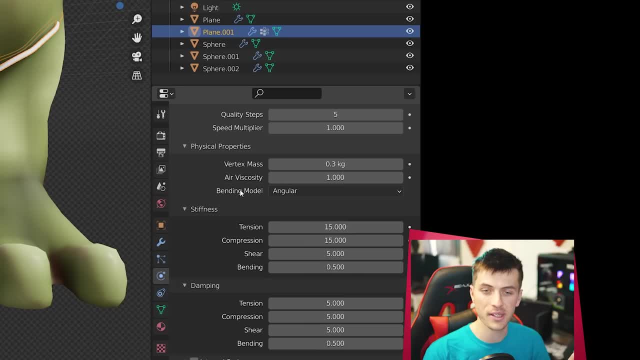 On this. I also added a quick cloth simulation Using the very basic settings And to make sure those pants don't fall down, You might want to add a quick weight paint map, Like I did here, Adding areas to the mesh that will be pinned. 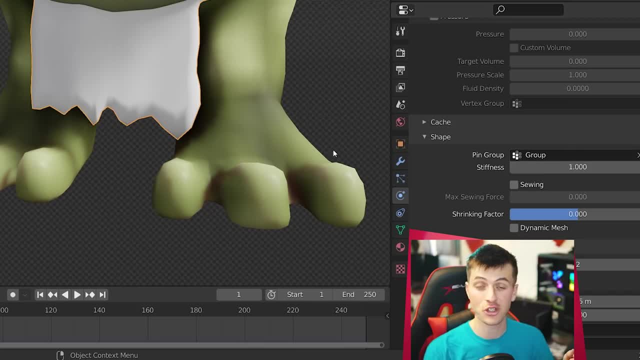 And then in the cloth settings All you have to do is grab that weight paint map that you created And choose that under the pin group. But having a little bit of moving fabric on your character Gives him a little bit of personality as well. 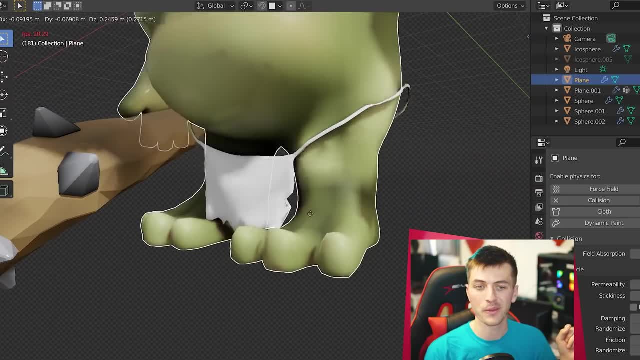 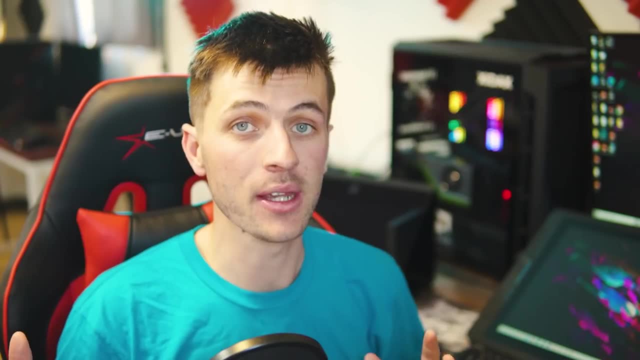 If you give your character the physics collisions, You can see that he now interacts with that cloth fabric And this is just kind of fun to play around with And gives it a more realistic simulation. But now you might want to bring your character to life with some basic animating. 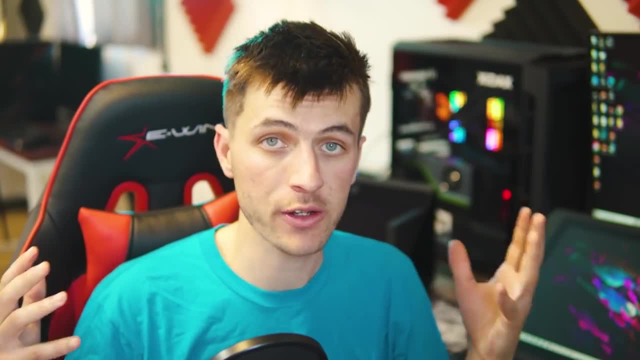 And to do this, you need to start by rigging your character. Now you can either create your own rig from scratch- I actually have a tutorial on that- Or you can grab a pre-made rig, Or use the add-on Rigify to add a rig to your character. 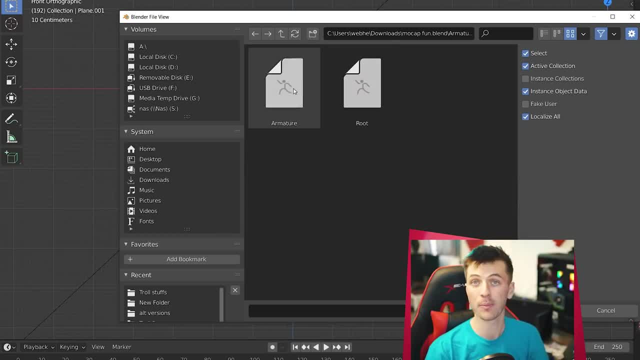 So for this, what I'm going to do Is I'm going to grab the rig that is used with my motion capture suit And I'm just going to import that into my blender file And, as you can see, We're going to have to work on the proportions a little bit. 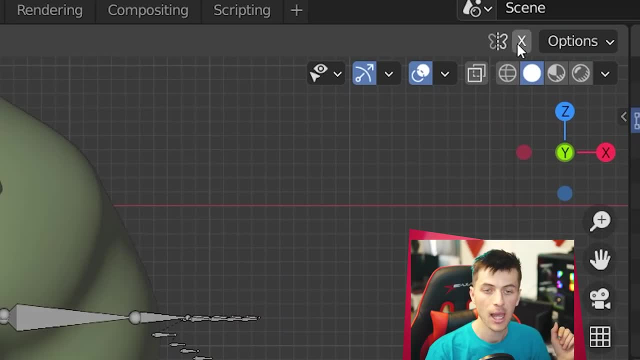 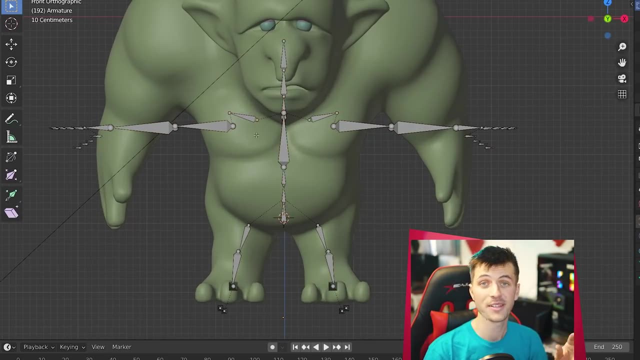 So just tabbing into edit mode And grabbing the X mirror option as well. to save time, I'm going to just position these bones over my character By moving them around quite a bit To make them fit the shape of this character, Jumping from front to side view. 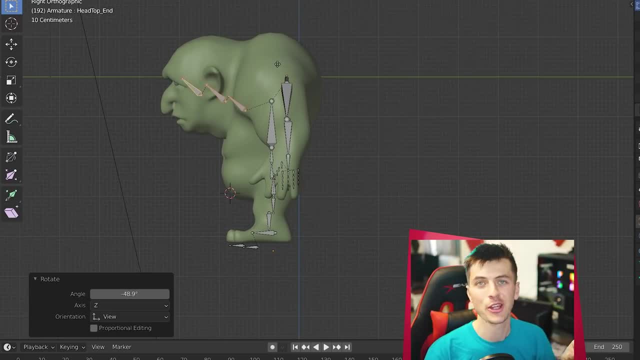 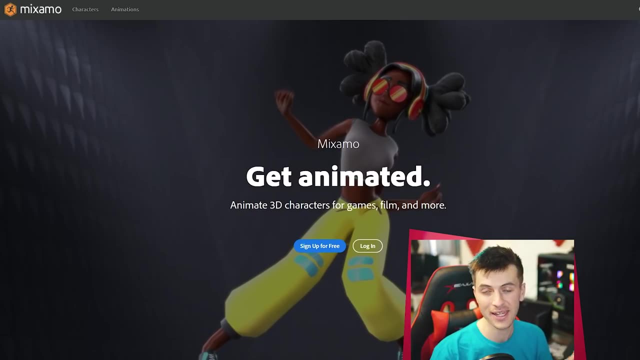 To make sure that these bones are actually inside my character From all views And then just to see how your character looks. You might want to throw some animation data at it. You can either animate your character by hand, Which might take a while. 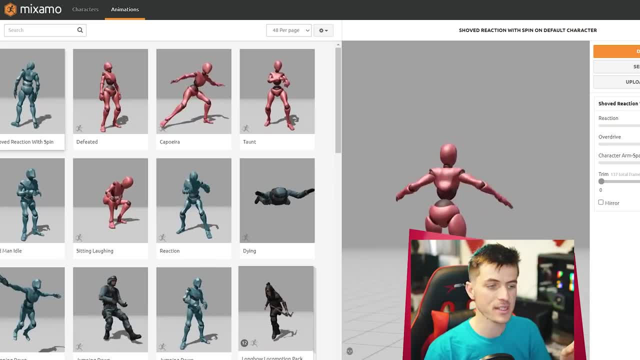 Or you can download animation data as an FBX file off the internet. Sites like Mixamo, I believe it's pronounced- Are great databases for a lot of animation data that you can download. Or if you have a motion capture suit, like I do, 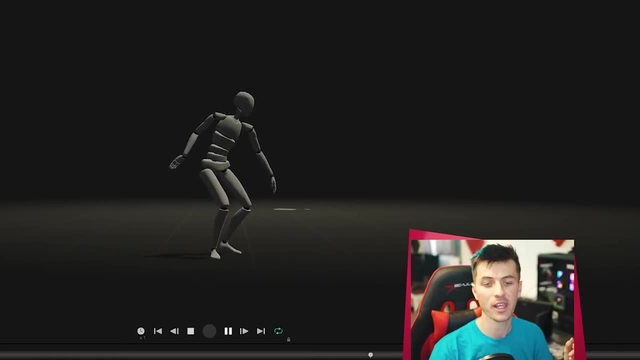 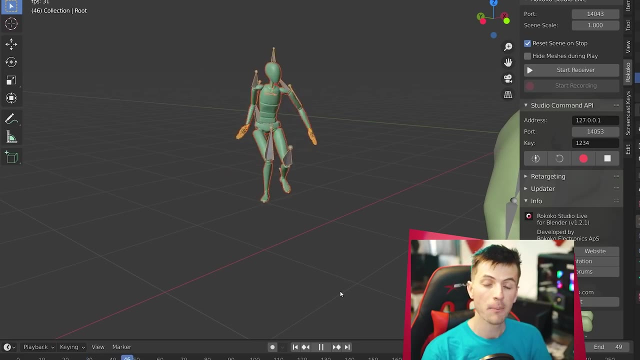 I'm just going to do my best: troll walking impersonation. Save out that animation data And then import it into my blender file As an FBX file. Of course, you'll then want to parent your character to your armature By going control P. 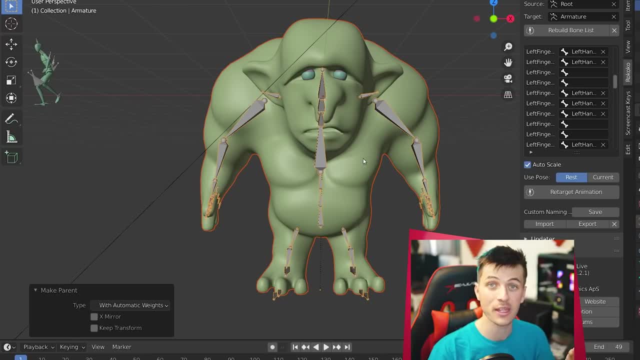 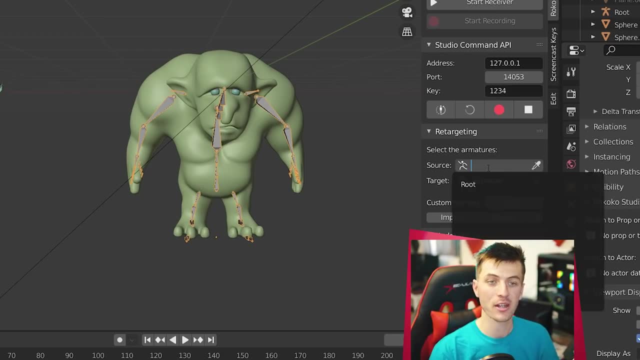 Using with automatic weights. You might have to tweak these weights a little bit In weight paint mode, But for the most part it actually works pretty good. Then I'm going to use the Rukoku studio app for blender. That allows me to map the animation data from one rig to another. 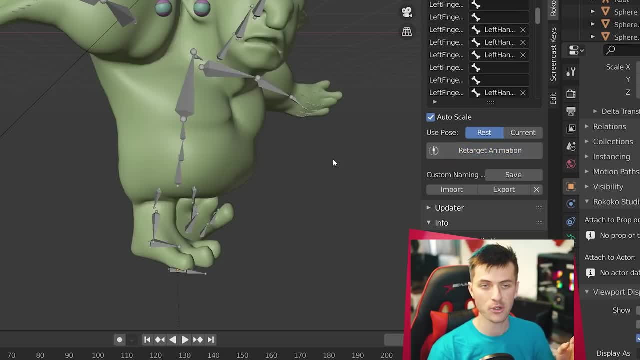 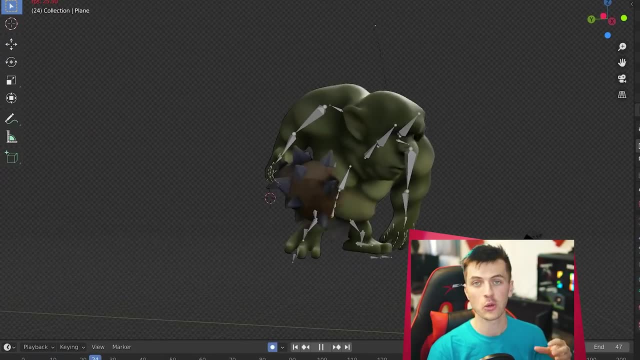 So just to see what it looks like animated, I can use the motion capture data that I captured And, with a few clicks, copy that animation data To my troll rig. now, Depending on how crazy your character is, You'll likely have to do a little bit of tweaking to the armature animation. 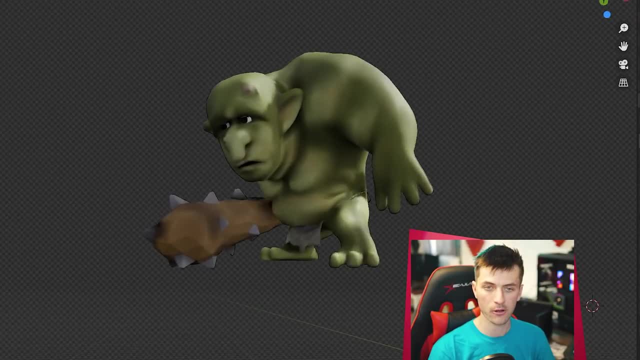 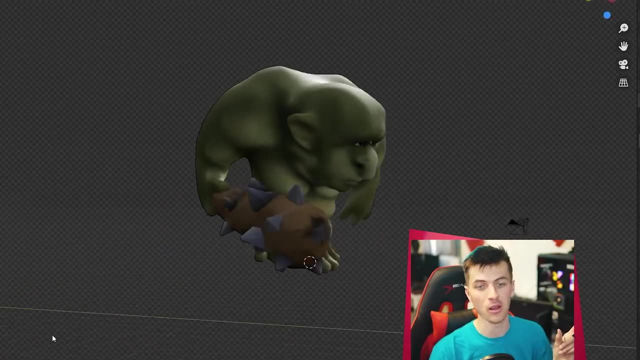 In the graph editor, But after I did a little bit of that, You can see that our character in motion Has been added, And that's essentially the entire process of character creation In a nutshell. But I hope you guys enjoyed the video. 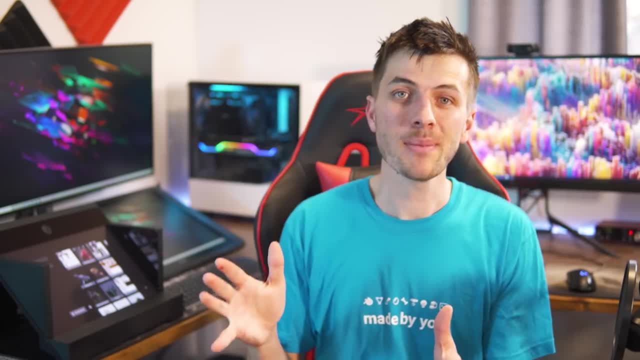 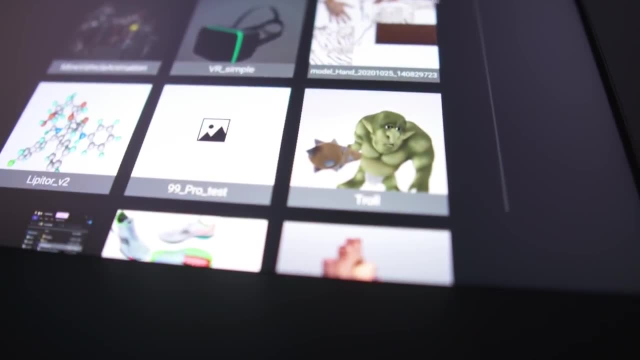 Learning sort of the process that goes into creating characters in blender, And had some fun along the way. But as promised at the beginning of the video, It's now time to demo our finished character On the Sony Spatial 3D display. You obviously can't capture it on camera. 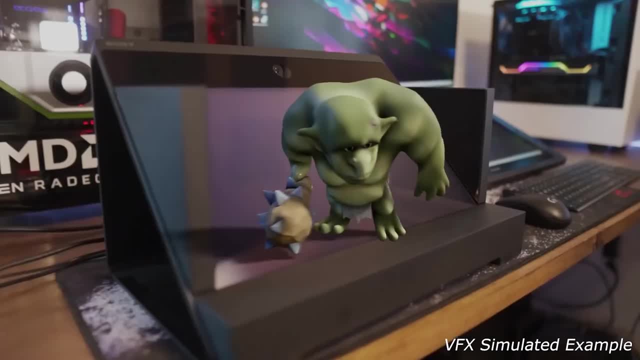 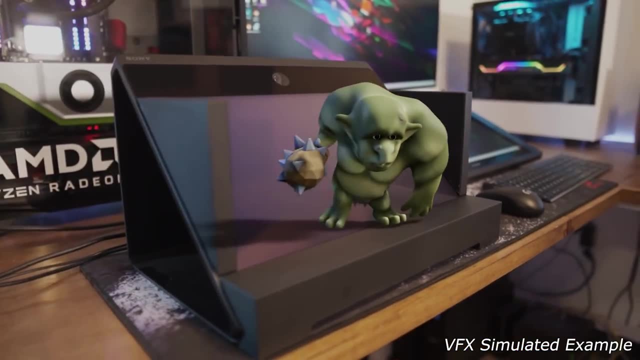 Because it's using advanced eye tracking To follow your eyes and update the frames immediately For whatever you're seeing. But here's a quick visual shot of what it essentially looks like to your eye And it's so cool. It honestly feels like your model is just sitting there in space. 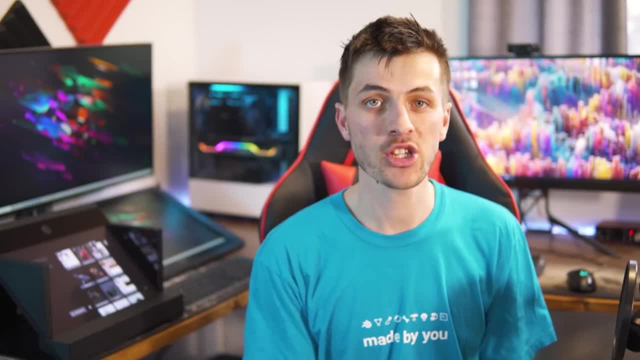 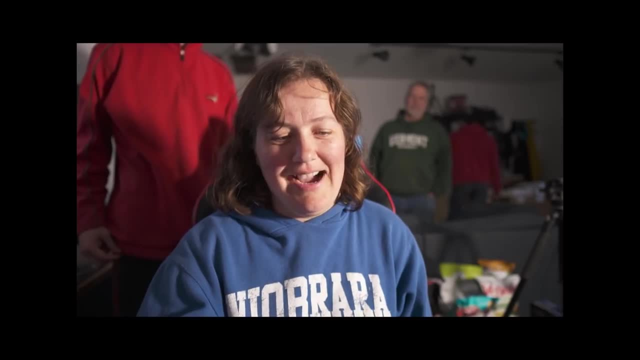 And you should be able to reach out and touch it. I've also captured some reactions From friends and family members To see what sort of reactions they have To a 3D display. So thanks again to MSI for sponsoring this video.